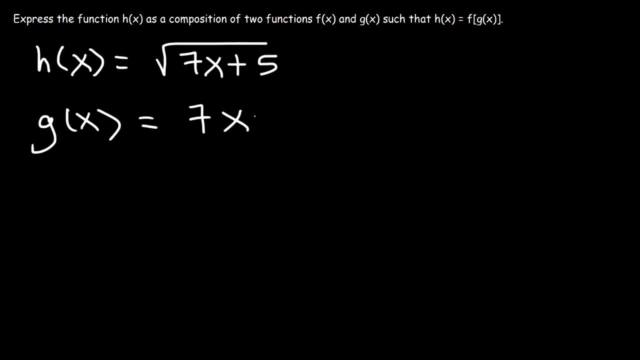 be g of x. The stuff on the outside is the square root symbol and that's going to be f of x. So f of x is the square root of x. So if we want to determine h of x, which is the composition of f and g, notice that if we take g and insert it into f, that is, if 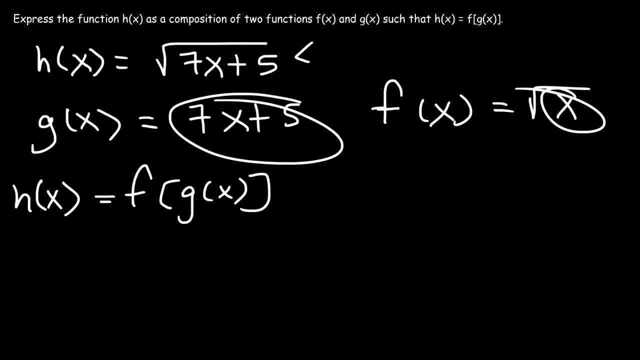 we replace this x with 7x plus 5, that will give us h of x. So here's the square root symbol, but without the x. So replace the x with 7x plus 5.. And that will give us the original function. But these are the answers that we're looking. 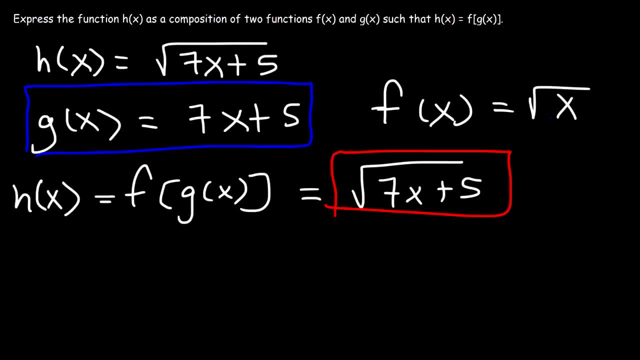 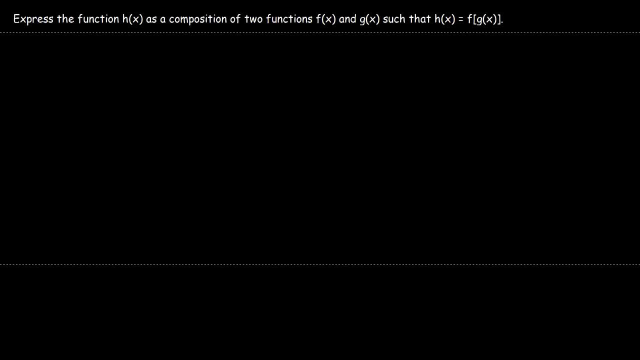 for g of x is 7x plus 5, and f of x is the square root of x. So let me give you another example that you can work on. So let's say that h of x is 1 divided by x plus 3.. Go ahead. 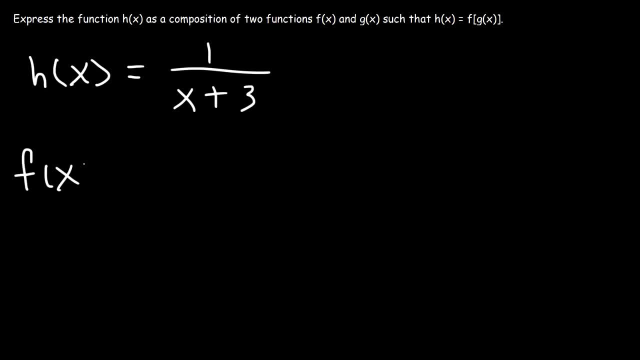 and look at the outside function f of x and also the inside function g of x. The outside function is going to be 1 over x. The inside function is simply x plus 3.. Because if you replace x with x plus 3, you're going to get 1 over x plus 3.. And that's pretty. 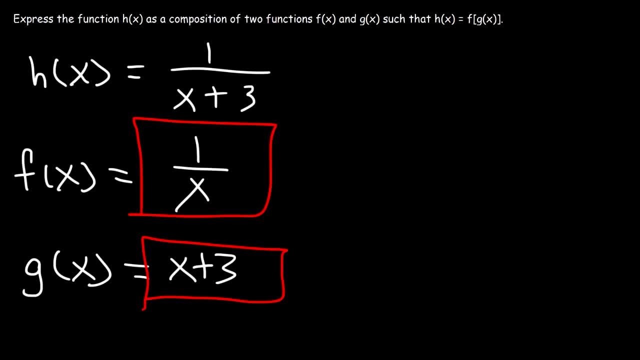 straightforward, So these problems are not too bad. Let's try another example. So what about this one? Let's say that h of x is the absolute value of 3x plus 2.. What's the outside function f of x and the inside function g of x? We can see that on the inside. 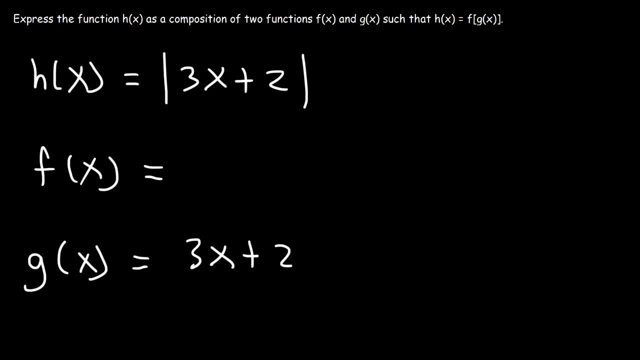 we have 3x plus 2.. So that's g of x. The outside is the absolute value of x, And that's it. And let's do one more example. Let's say that h of x is 2x cubed plus 7x minus 3 raised. 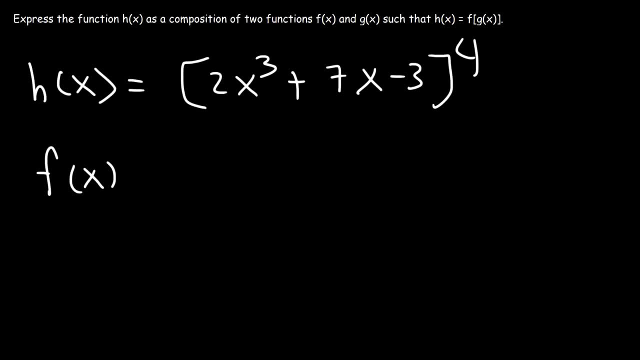 to the fourth power. So what's the outside function f of x and the inside function g of x? On the outside it's x to the fourth power, On the inside, 2x cubed plus 7x minus.